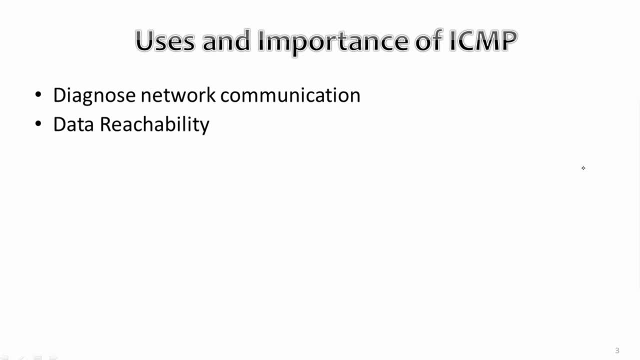 intended destination in a timely manner. Commonly, ICMP Protocol is used on Network devices such as Router PCs Switches, Since ICMP is a crucial for error reporting and testing, but it can be also used in DOS attacks. ICMP has no ports and is either TCP or UDP, but it has Types and Codes. 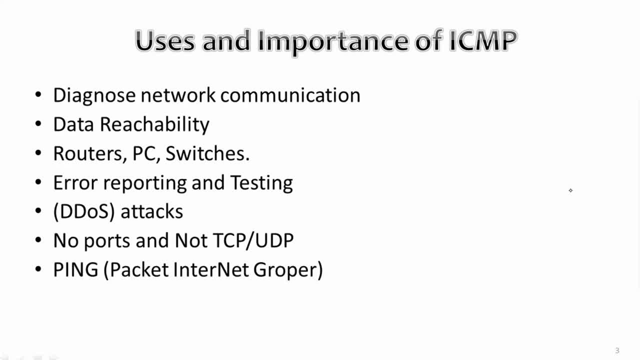 ICMP is better known as Ping. Another important use of ICMP protocol is to know the IP address with which it is being sent to the server. ICMP is also known as Ping. Another important use of ICMP protocol is to know the IP address and ping. Another important use of ICMP protocol is to know the IP address with which it is sent to the server. 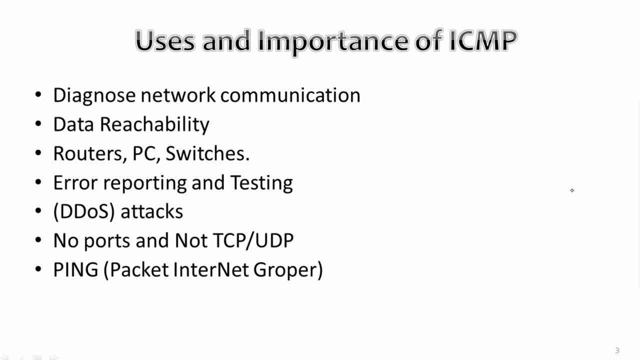 ICMP protocol is used to perform network diagnosis by making use of traceroute and ping utility. So traceroute basically used to know the route between two devices connected over the internet, where ping is known as the echo request message as it is used to measure the time taken by. 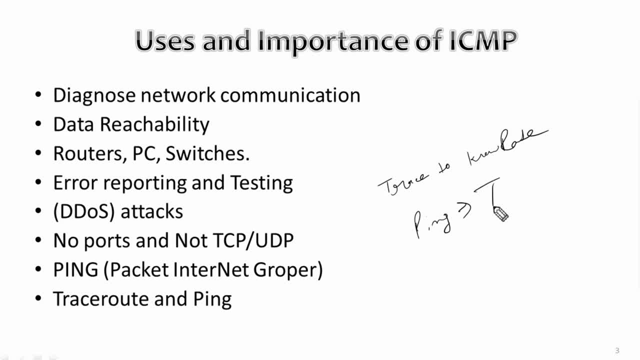 data to reach the destination and return to the source, So these replies are also known as echo replies messages. If you would like to know more about the ping and traceroute, we have already uploaded the video. you can visit the channel page and we will also put the video link in the description. 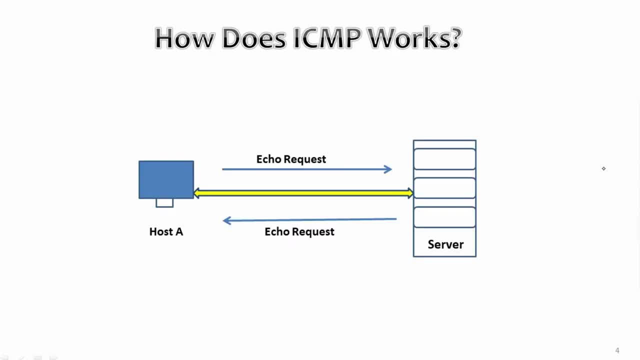 Moving on. so now let's understand how ICMP work. First, ICMP is the primary and important protocol of the IP soup. But ICMP is not associated with any transport layer protocol which is TCP or UDP protocol. That's why it does not need to establish a connection with the destination devices. 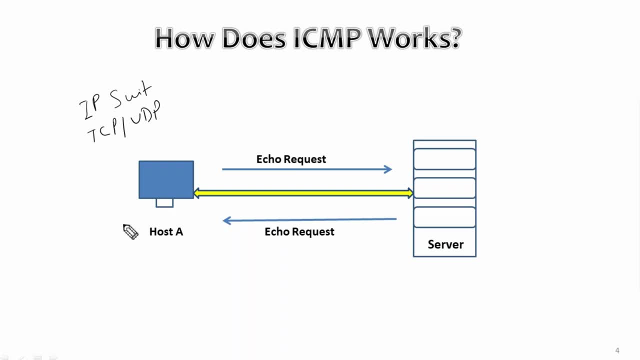 Before sending any message. it is a connectionless protocol. The working of ICMP is just being associated with TCP, as TCP is a connection oriented protocol whereas ICMP is a connectionless protocol. So whenever a connection is established before the message sending, Both devices must be ready through a TCP handset. and to know more about TCP handset, we have 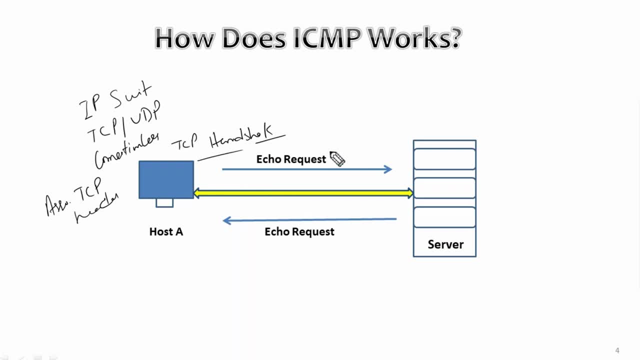 already uploaded video and we will share the link in description or you can also visit the channel page Moving on. so these ICMP packets are transmitted in the form of datagram that contain an IP header with ICMP data. So ICMP datagram is similar to a packet, which is an independent data entity. 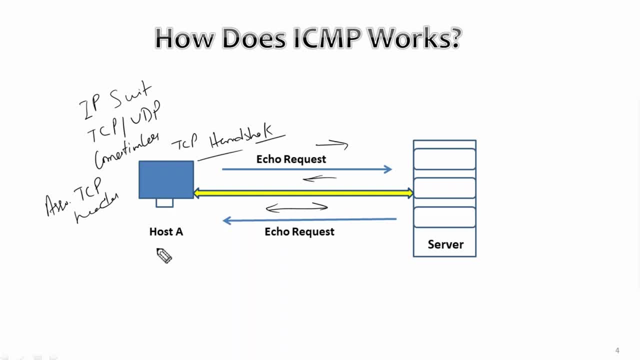 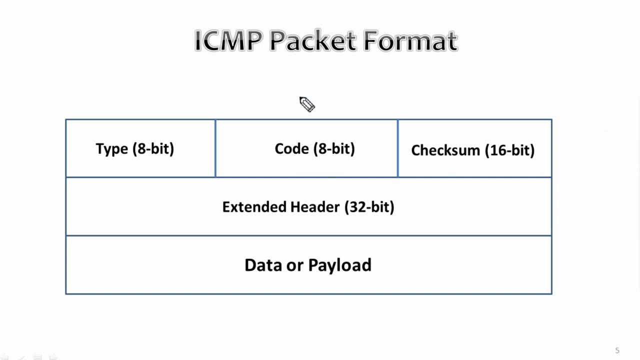 So this is an independent data entity In the header and this is how ICMP being used between the source and destination devices. Now let's moving on and look into the ICMP packet format also. In ICMP packet first, 32 bit contains three major fields, which is type, code and checksum. 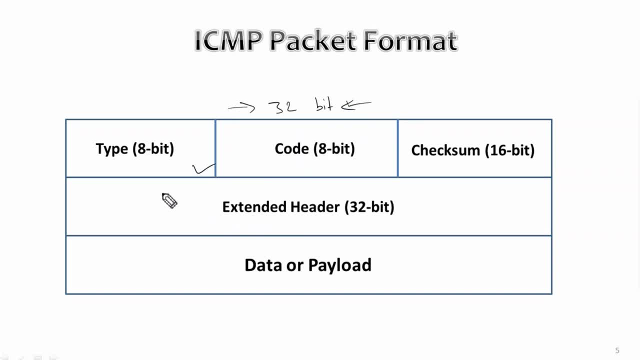 First, this type, the initial 8 bit of the packet, is for message type. it provide a brief description of the message So that Receiving network would know that kind of message it is receiving and how it respond to it. Here are some common messages types like type 0, which is echo reply, type 3, which is destination. 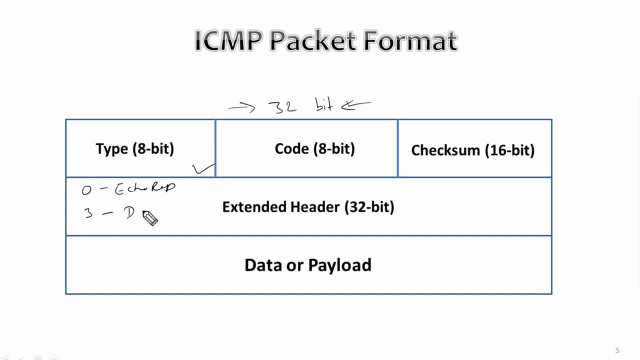 unreachable. type 3 means read redirect message, type 8 means echo request, type 11 means time exceeded and type 12 means parameter problem. Then we have another field, which is code. This is also 8 bit. code is the another 8 bit in the ICMP packet format. and this field. 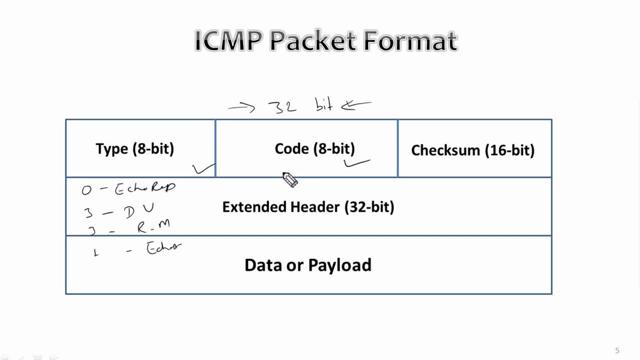 carries some additional information about the error message and type. Then we have checksum. So checksum, the last 16 bit, are for the this field and in ICMP packet header the checksum is used to check the number of bits of the complete message and enable the ICMP tool. 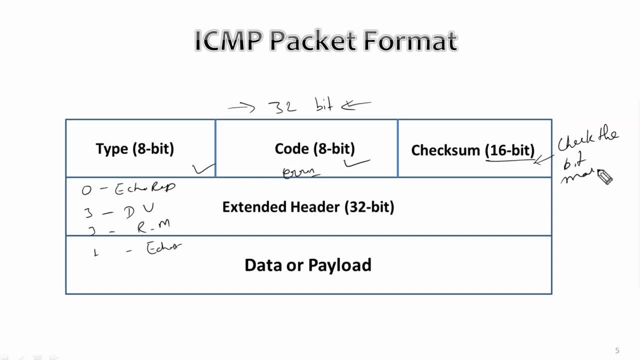 to ensure that complete data is delivered. This field is used to check the number of bits of the complete message and enable the ICMP tool to ensure that complete data is delivered. Then we have these two: extended header and data or payload. So extended header is also 32 bit of the ICMP header and which has the network of pointing. 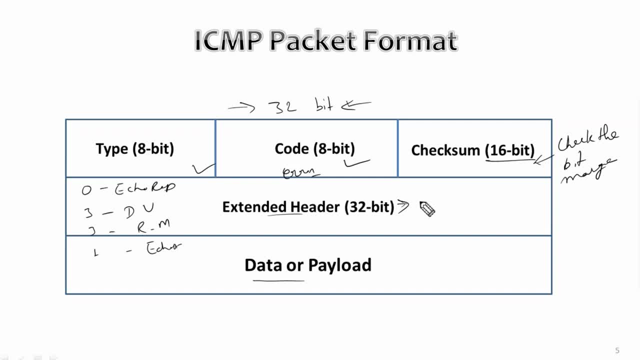 out the problem in IP messages, Then the data or payload. So this last part of the ICMP packet is a variable length, having a variable length, and the byte include in IPv4, IP protocol version 4.. It has 576 bytes And in IPv4.. 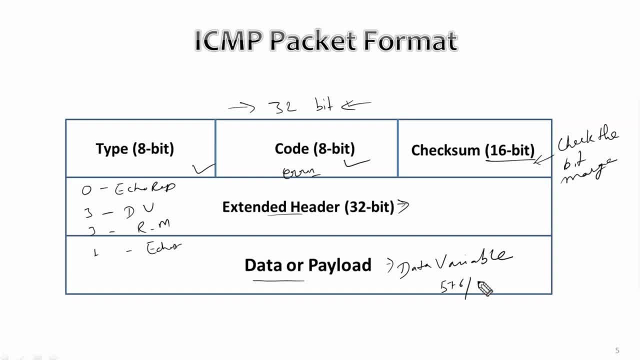 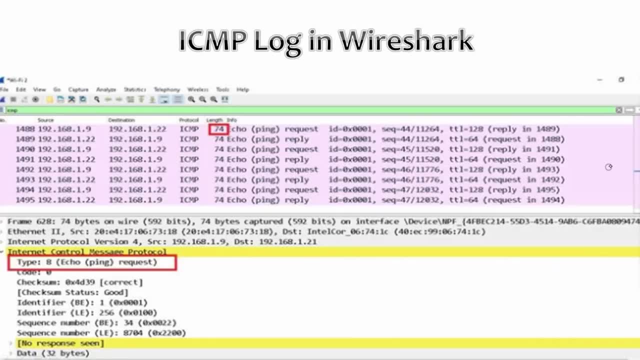 And in IPv6 it has 1280 bytes. So moving on now. this is a Wireshark capture of ICMP log and you can see on the screen it has ICMP type code checksum. above you can see the length, the request and reply messages type, then protocol. 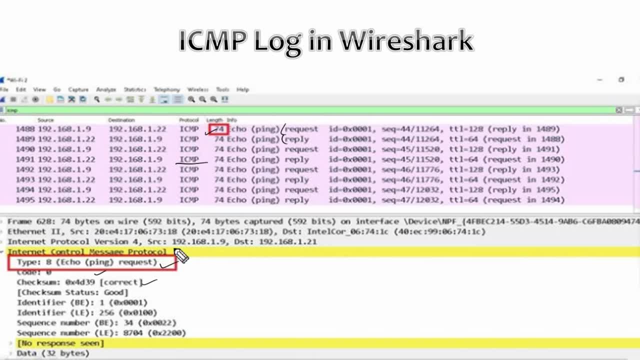 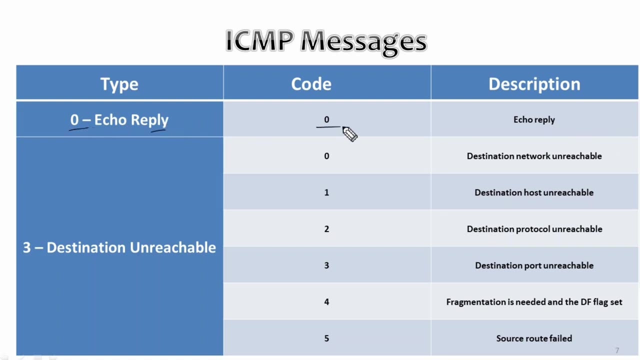 So this is how we can identify an ICMP log in the Wireshark check. Moving on, So let's look into some The Integrity of ICMP messages First. we have Zero echo reply That the code is still zero and thus this is. it is a eco reply. 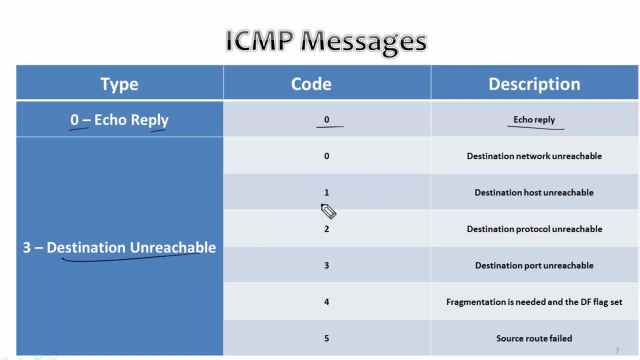 Then we have the destination unreachable. When we are receiving destination unreachable and the code is zero, This means destination network is unreachable. When the code is one, this means destination host is unreachable. When code is two, means destination protocol is unreachable. So now this is the code. 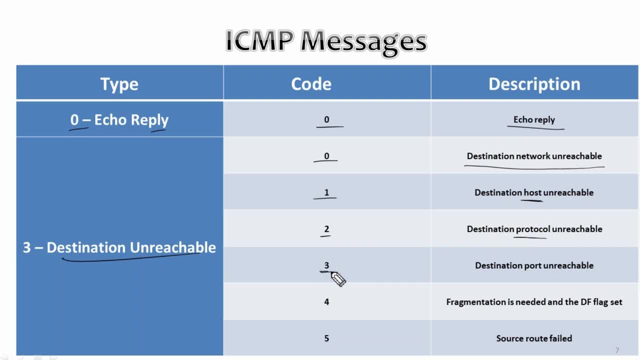 This is the node. when the code is three, that means destination port is unreachable, and when the code is four means fragmentation is needed and the df flag is set. if the code is five, then it says source route failed. so this is how we can identify based on the code of the messages. then we have the redirect. 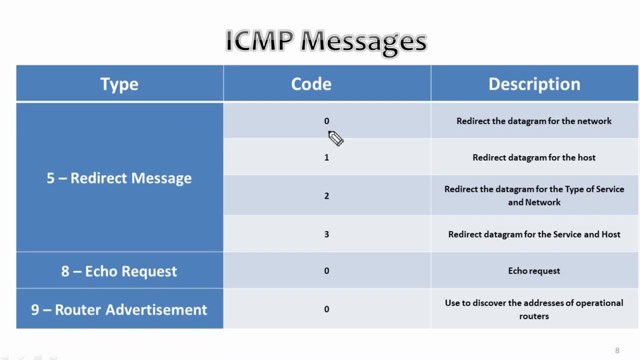 message. so if the redirect message is set as 0 means it redirects the datagram for the network, and when the redirect message set as 1 means it redirects datagram for the host, then we have the echo request. no, sorry, this is still from. so when the redirect message set as code to means here: 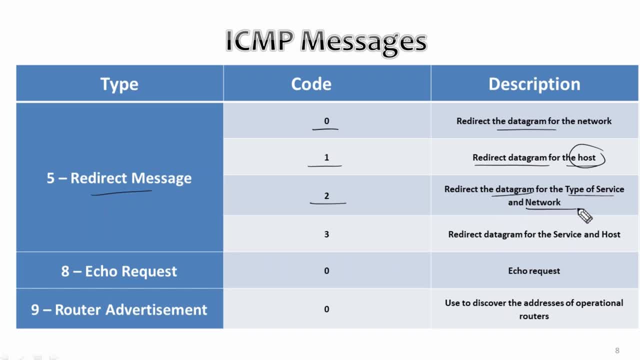 you the datagram for the type of service and network. when the redirect message set as 3, that means redirect datagram for the service and host also. then we get the echo request. that is the code 0 and it will be for the echo request. then we have the route advertisement for which we will get also. 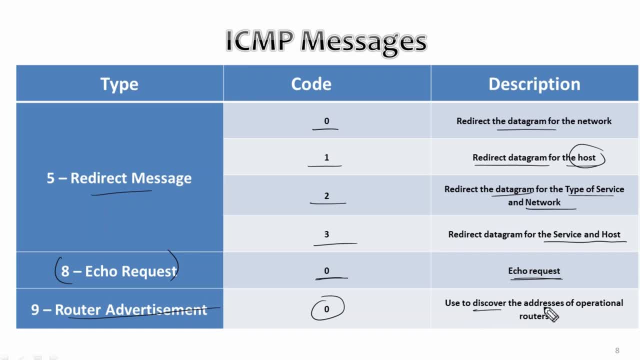 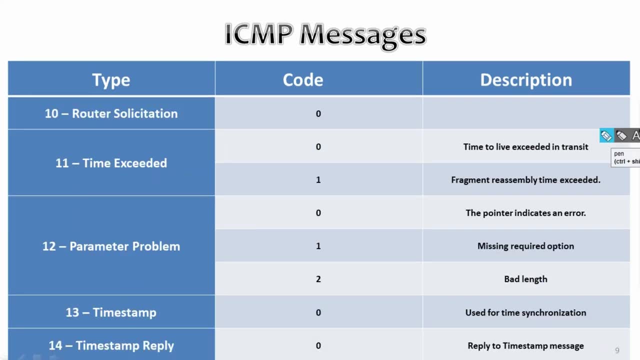 code 0 and that used to discover the address of operational routers. then we have the time exceed. so when time exceeds set as 0, that means the ttl exceeded in transit. then time exceed is set as 1, that means fragment assembly time exceeded. also later we have the parameter problem. so this: if